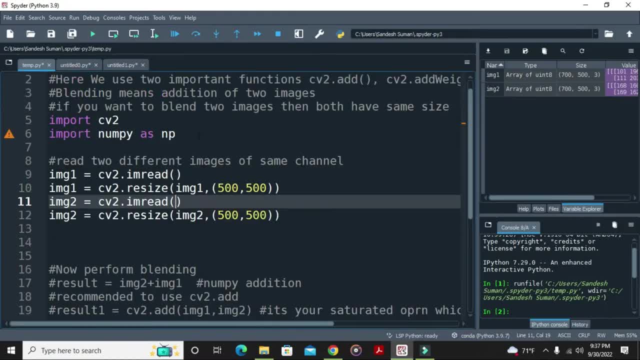 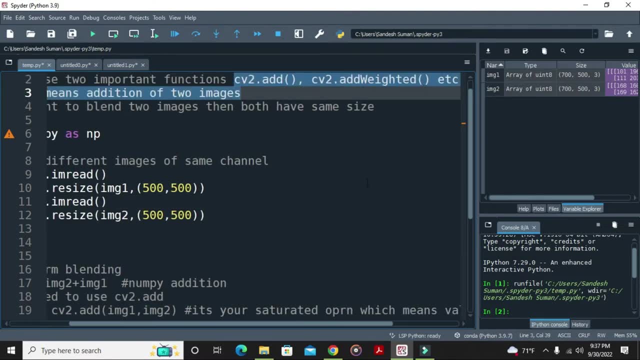 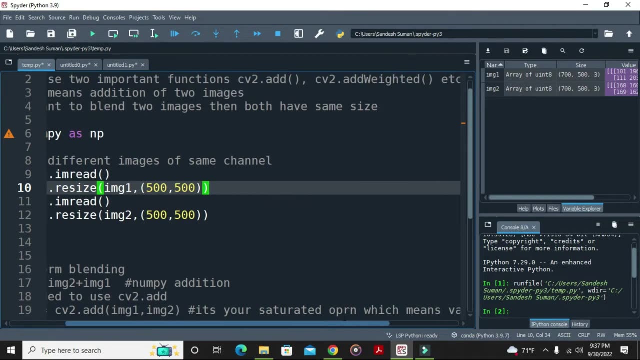 so let's directly go on our id and see what's the code. so actually, you see that we have two important functions, which is cv2.add and cv2.add- weight for blending the two images images, right? so blending means addition of two images, so it's actually see the 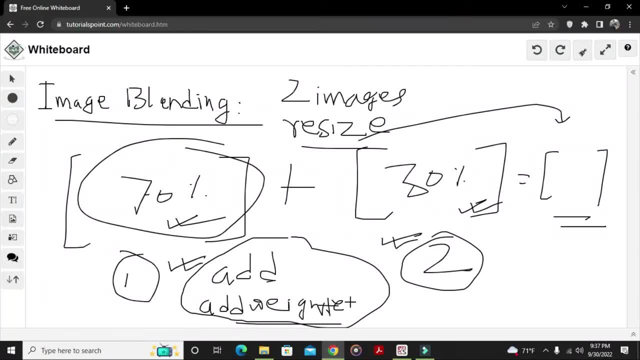 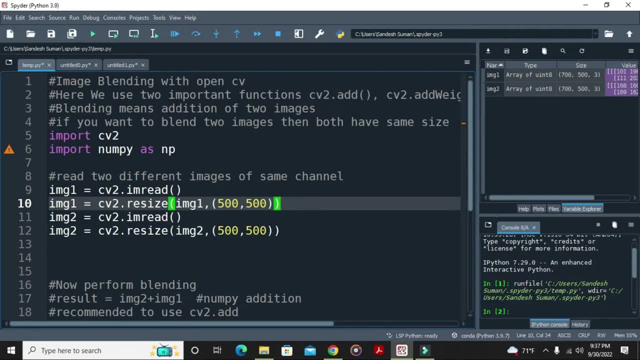 function is add weighted. so you can see: just add. you add weighted. so that is what the functions are. and so blending simply means that you add your two images, and if you want to blend your two images, then you and the both of the images should have the same size, as we already know that. so now let's import. 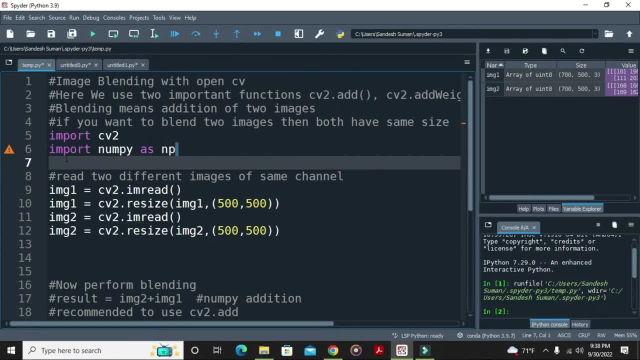 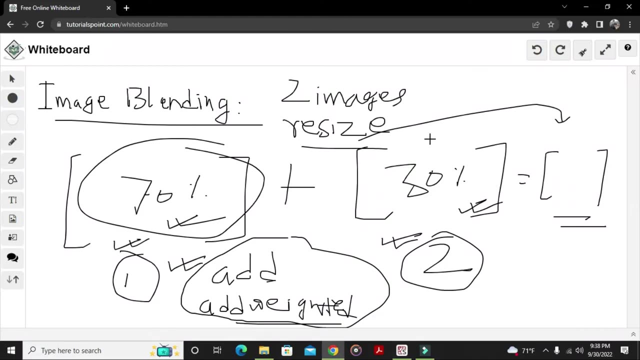 our cv2 library, which is the open cv library, and we have imported our numpy as np, since if the numpy addition since image is numpy array, so for numpy addition we have imported the numpy library as well. now what we do is that we read two different images of same channel. now the first thing you need to 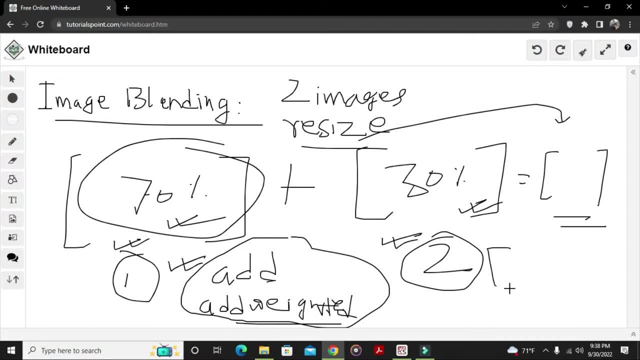 know is that your channel should be equal means that you need to add any two color values, two color images, since color image have a channel of three. so you are adding images of equal channel but then you cannot add in image which is of color image with a black and white. 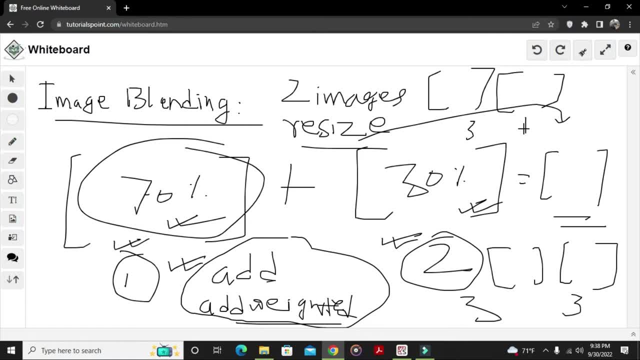 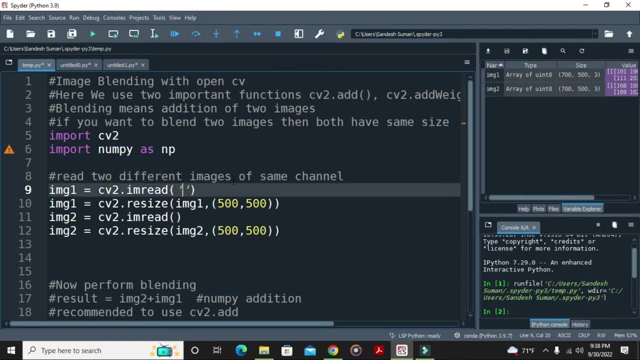 pixels. I mean to say that you cannot add a gray scale image and a color image, since both of them have unequal channel value. now let's go and have our first image. so I already have my images here. so you just go and extract the path of your image in a string and let's go and give the 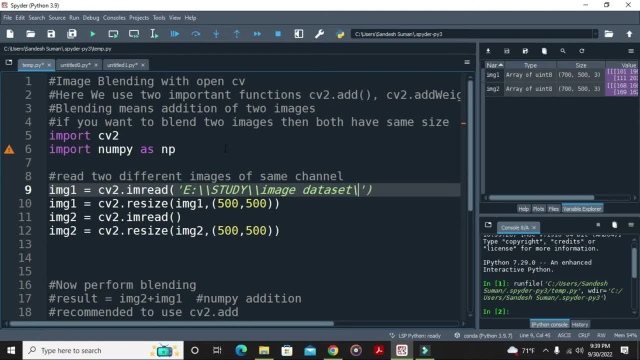 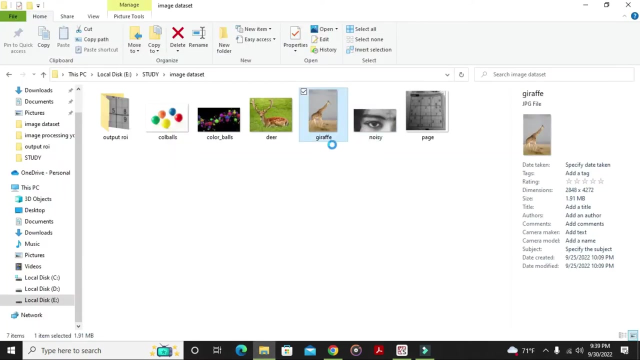 double. go there and go and just write the name of the image. so my first image is of deer and my second image is off, set off. so let me just go and copy that jirafjpg. so let me cross check my spelling: J-R-A-F-F-E. okay, so this one is correct. now what I do is that I am gonna resize. 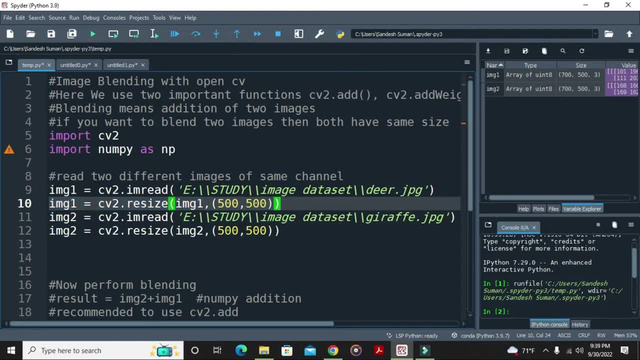 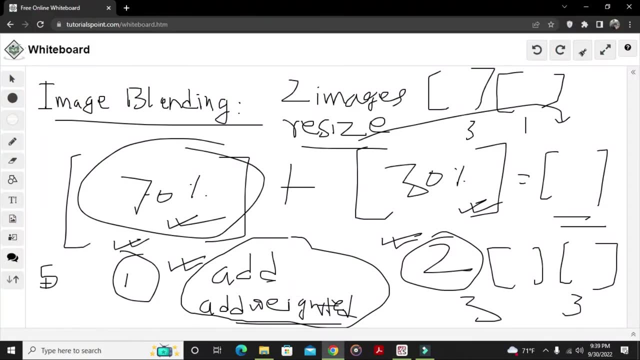 both of them, so I am going to resize both of them. so I am going to resize both of them into equal size. so what I have done is that, for my image 1, I have used the resize function to resize it into 500 comma. 500 means that 500 is my width and 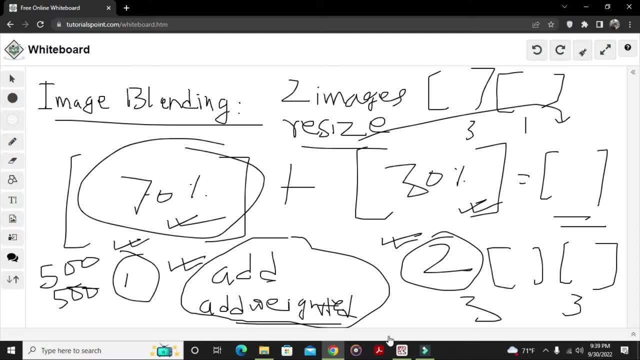 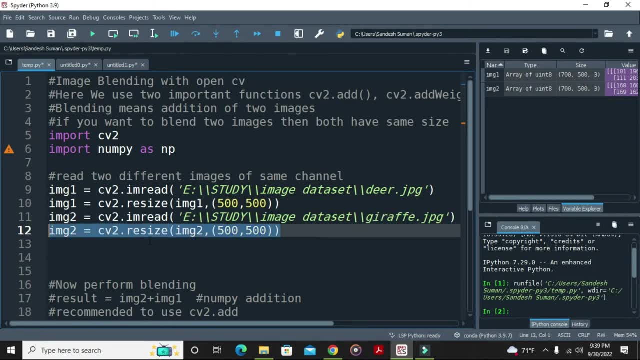 500 is my height, so I have resized them onto equal size. now, once I do that, I again go to image 2 and read that, and then I again resize my image 2 into a fixed width and height of 500 comma 500. now, since both of my images have equal, 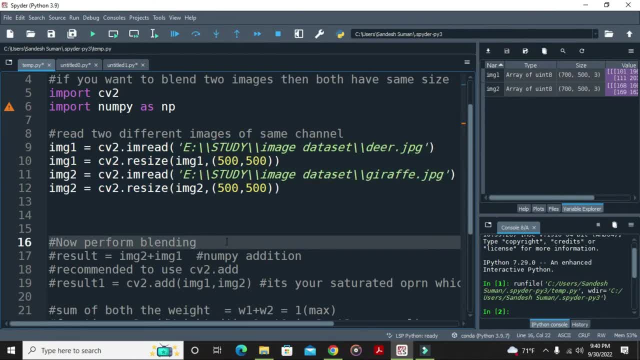 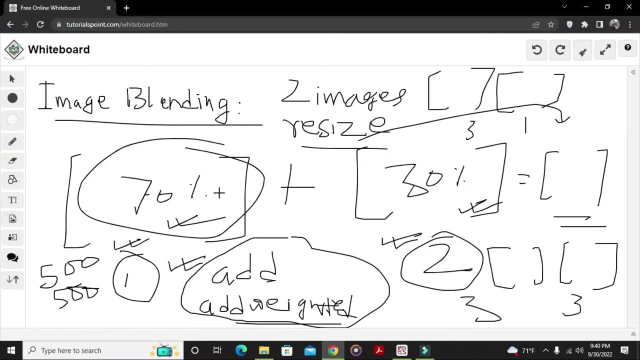 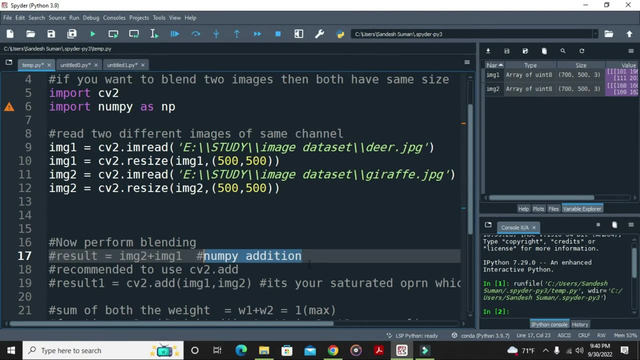 size. now it's good to go for performing the blending. so this first simple thing is that you can just go and add. the numpy addition means that it will go and just add the pixel values of both of it, I mean the array of it, right, the elements of the array, but that array is called as what? 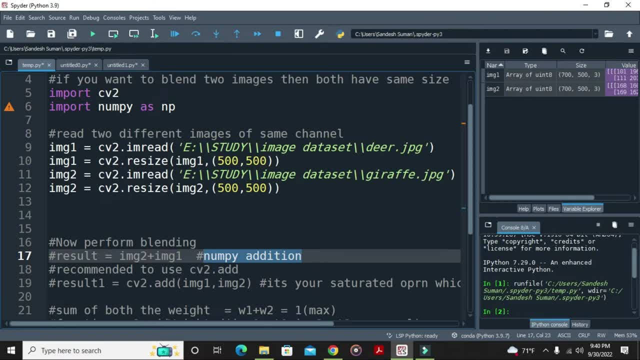 pixels, right, so it simply adds the pixels. so let's go and have a look on our result. so result is simply image 2 plus image 1. now one thing you should be noting: that image 1 plus image 2 or image 2 plus image 1, both of them are. 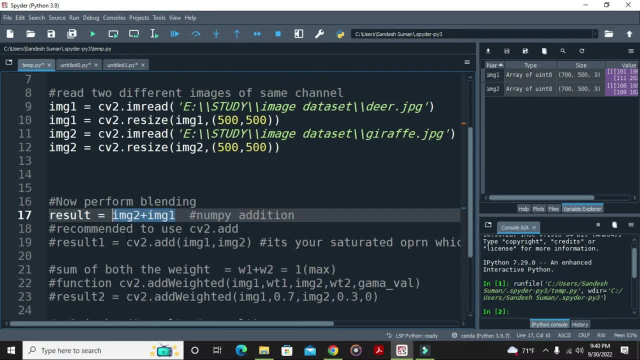 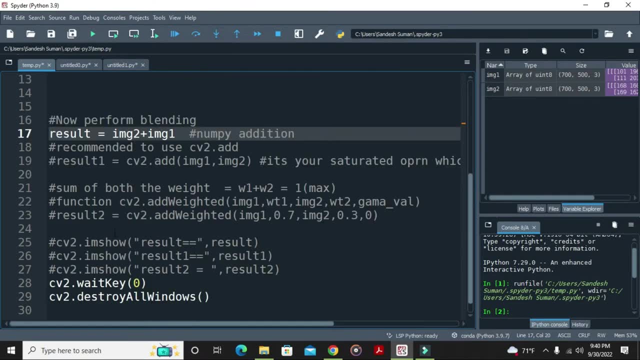 same thing. you won't find any difference in the output itself. so let's go and view the result. actually, what happens if you obtain the result of image 2 plus image 1, and how does it look like? so for that I am just going to use my mshow function, which is stored in the windows theme as result, and I am 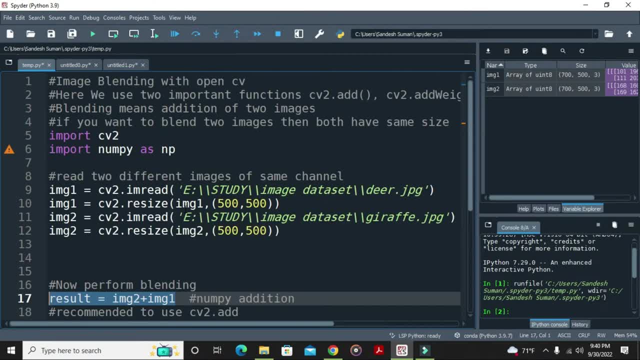 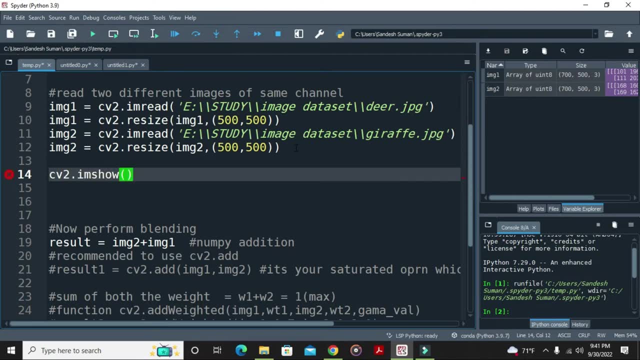 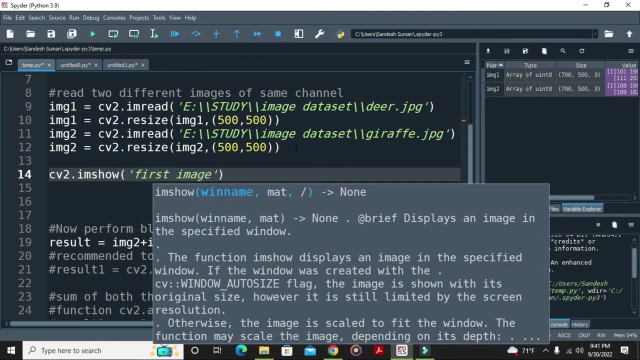 passing the result variable, which is storing my image 2 plus image 1. before that, let's go and just view our original images as well, so I'm gonna mshow that. so my first image right, first image or, and then pass image 1 and let's do. 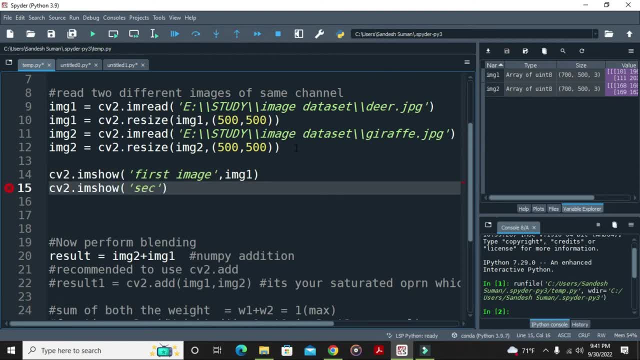 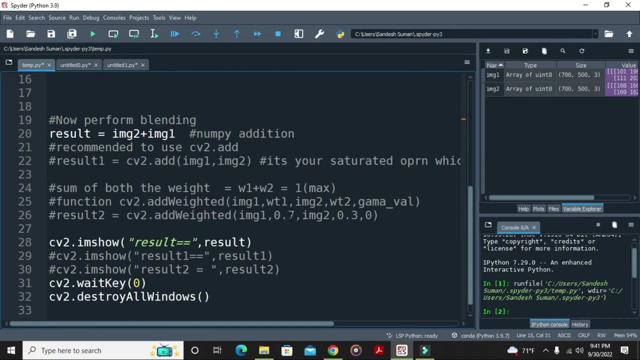 cv2.imshow my second image. so this is what I have done. I've just gone and added- I mean displayed by image 1 and image 2- so so that it would be easy for us to compare the output. so now let's just go and see how it looks like and 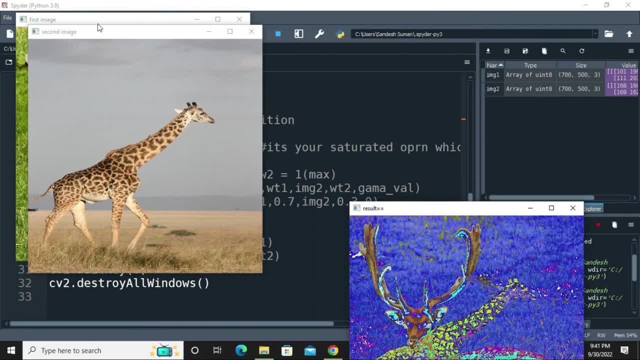 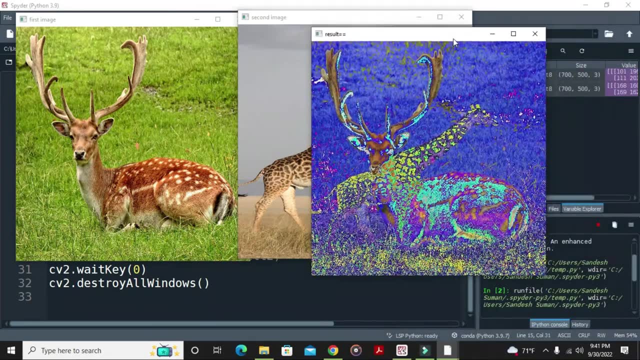 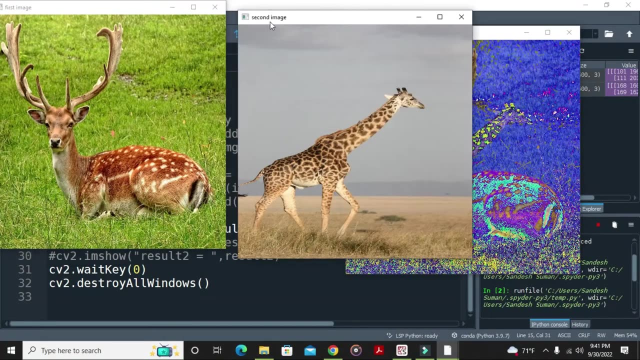 hit the run button and let's see what sort of image are you getting. so, yeah, this one is basically your first image and this one is the second image. now, the moment I added the pixel values of each of it, you see an image like this one right, so you can notice both the deer and giraffe in the picture here. so you, 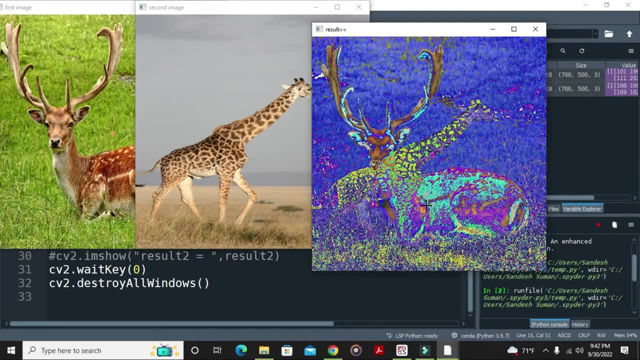 can notice that this is a kind of output you get when you just simply add two images. now, this has done what this is actually: added the pixel values of both images, image one and image two, and this is what you call the output. right, so your adding function. 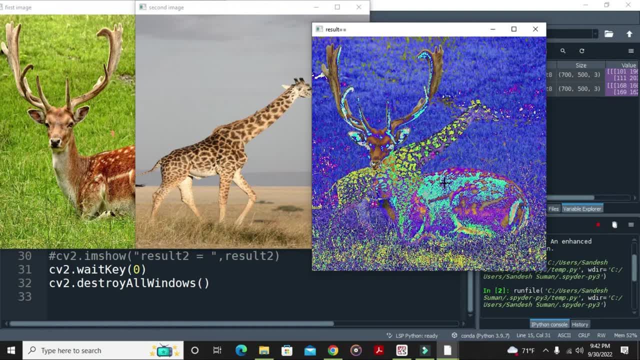 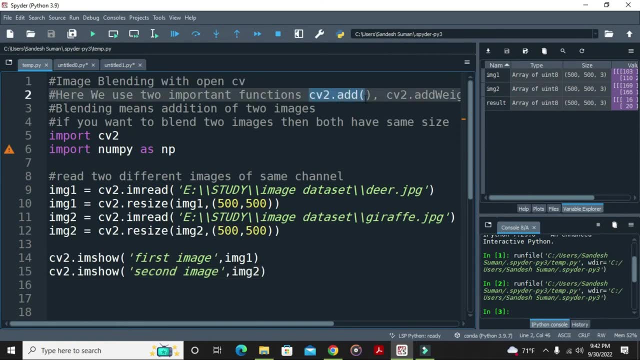 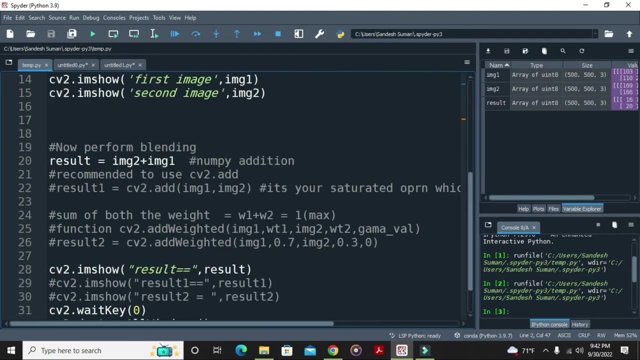 just adding. adding the two images just simply adds your pixel values. now let's go and have a look that what these functions are going to do: cv2.add and cv2.add- weight. so for that you have, uh, cv2.add, right, so you just need to use cv2.add and then just image. 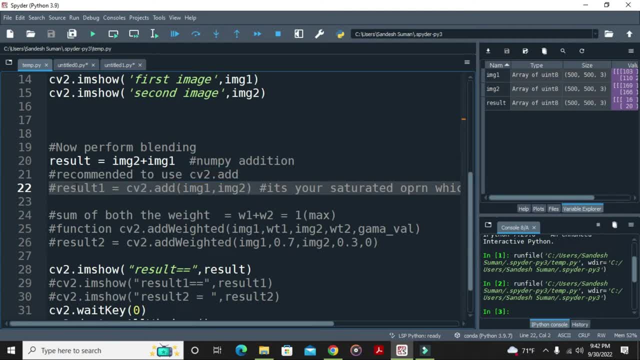 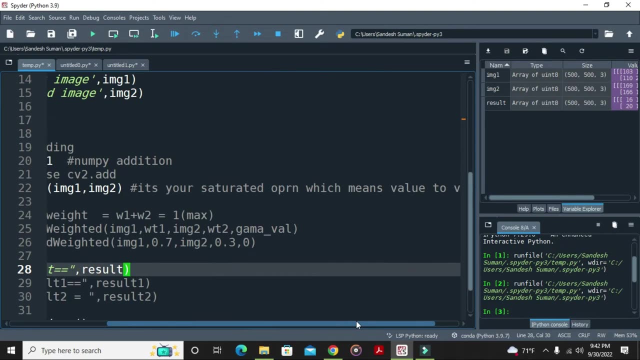 one and image two. uh, now it's uh. the result will be same if you pass image to an image one as well. so let me just comment this out, or let it be so: cv2.add image one in image two. it means that it will add, based on the saturation, right saturation. it will be adding your uh value to value based on. 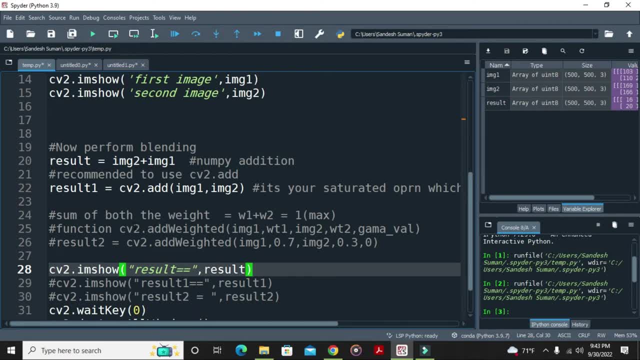 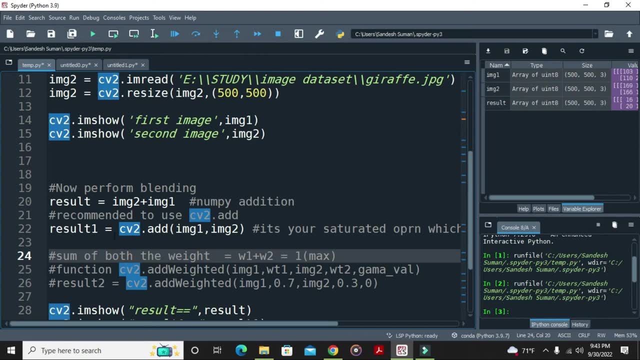 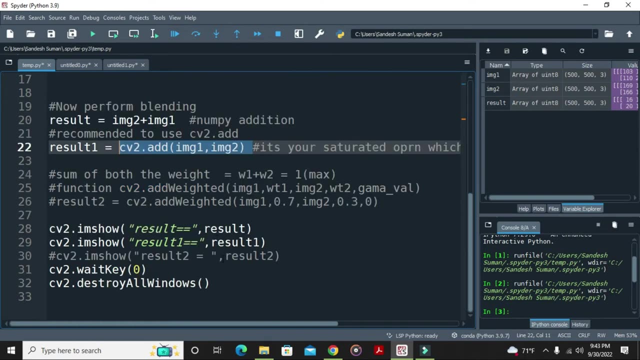 the saturation of the pixels means the intensity of both of it. now i go and i view my result, one, uh, which is stored in this, which is storing the value of cv2.add, adding of intensities of image one and image two, and let's have a look on how does it look now? so yeah, you can see that. 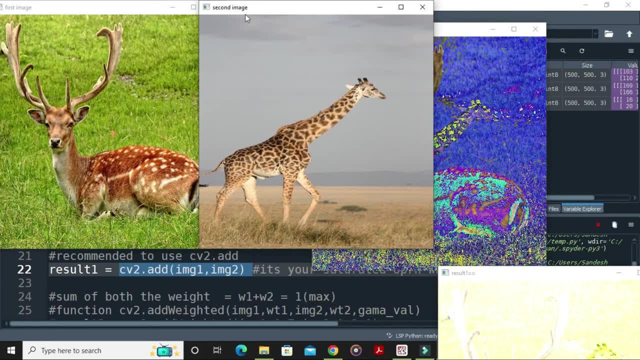 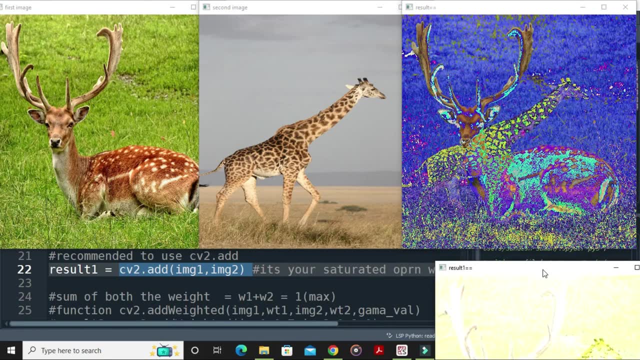 this one was your image one, this one is image two and this one was when we added both the images, just based on the pixel values. but then we have used this function, which is cv dot add, which actually adds based on the saturation point. so this is what the output you are getting. 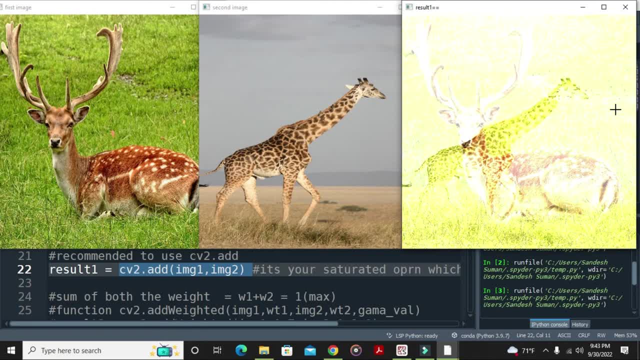 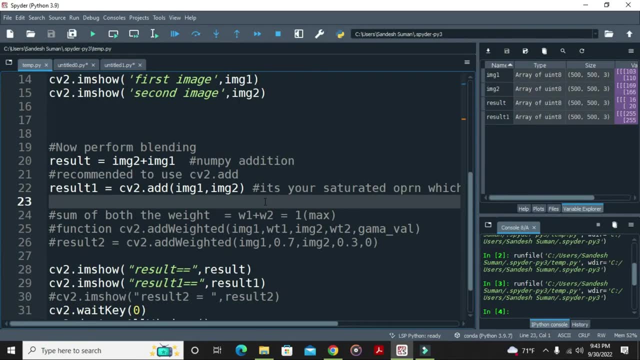 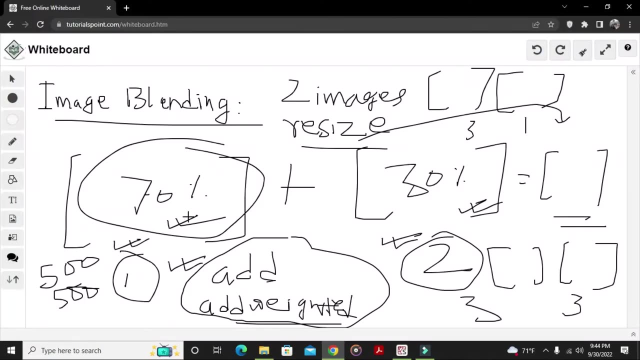 so you can see, you get an output like this. so what does this do? is that it has basically added both the pixels based on their intensities or saturation. now we have another function, which is cv2.add weight. so, as i already told you, that add weight means assigning certain weight to our 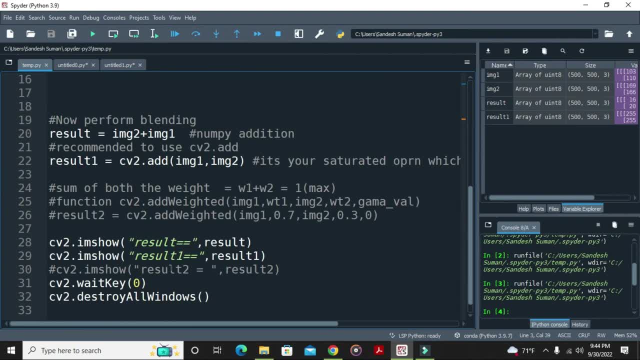 image. so what i have done is that i have gone and i have just used this function, which is cv2.add. right, i have passed the image one and i have passed 0.7. here means that 70 of image one, and 0.3, which means 70 of image two. and this one is zero, is the gamma value. so gamma value is. 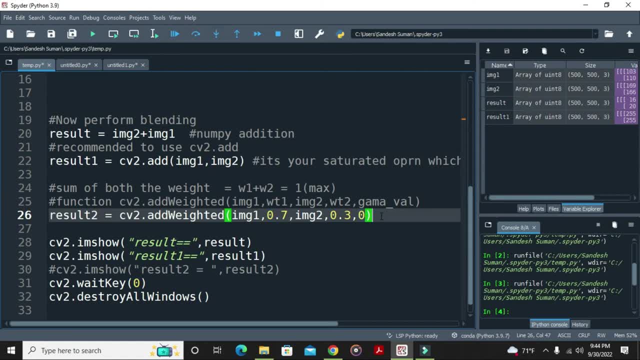 recommended to be zero, or you can also put it like one, two and three, but it's recommended that your gamma value should be passed as zero. so one thing: you might notice that your sum of both the weight should be equal to one. it means the maximum should be one. so in my case, 0.7 plus 0.3 is actually. 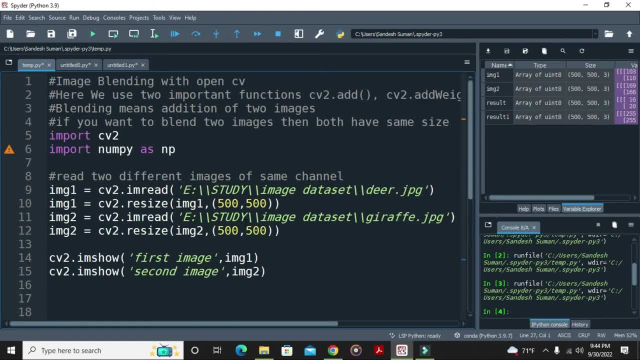 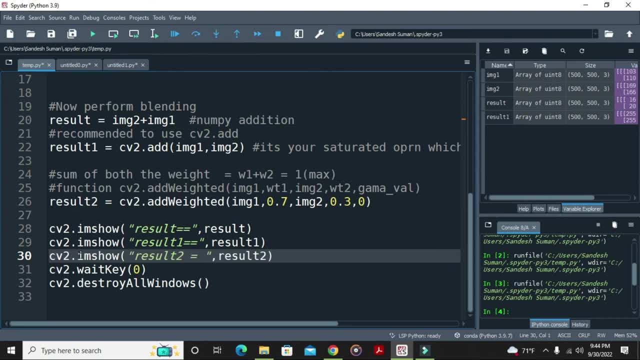 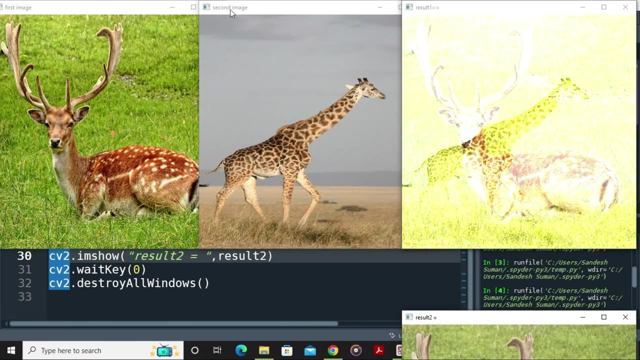 one. so it means that your first image will be dominant as compared to the second one. so now let's go and have a look on to our add weight output. so notice multiple of it, right? so this one is the first image. this one is second image. this is cv2.add, this is cv2. i mean, this is simply. 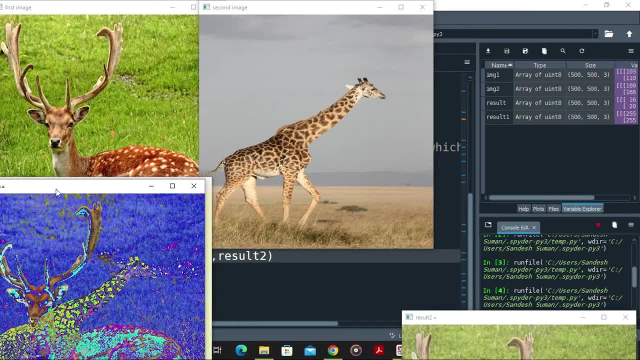 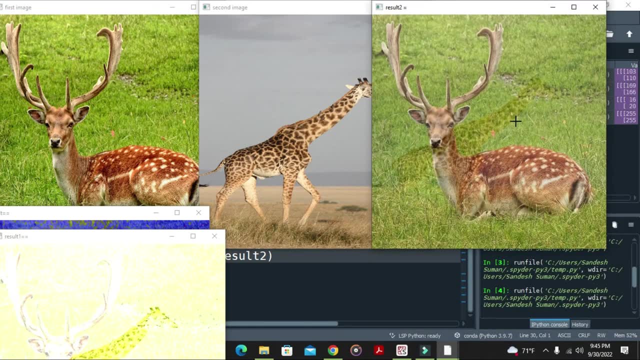 adding the two images based on the pixel values. now, what i have done is that i have actually added both of it using the pixel value, so you can notice that my first image is dominant and the second image you can see a slight view of it. since i've already passed 30 percent of, i've assigned 30 percent of weight. 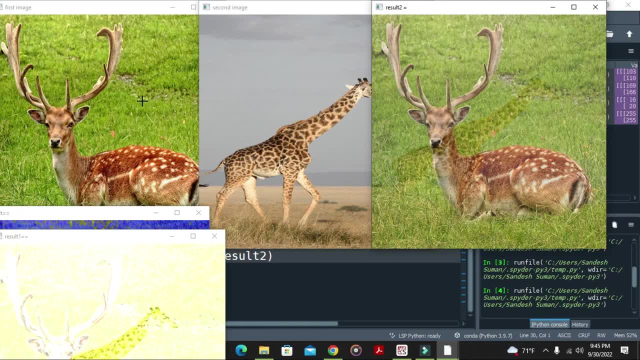 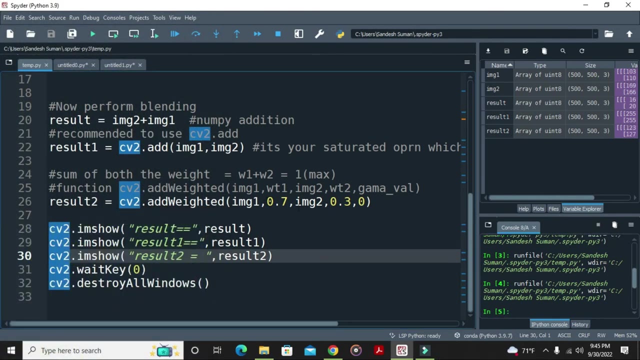 i mean 0.3 of it and then 0.7 of it, right? so, uh, you can basically notice that the intensity of my first image is more as compared to that of second. now let's just try and look, uh, reverse the order and then just view our output. so, if i 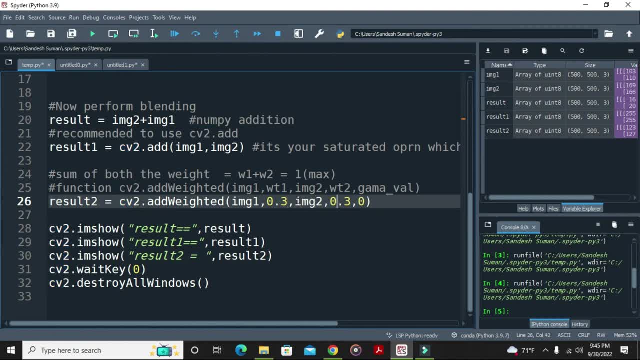 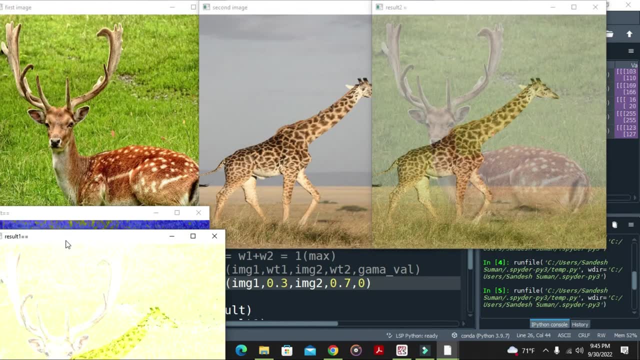 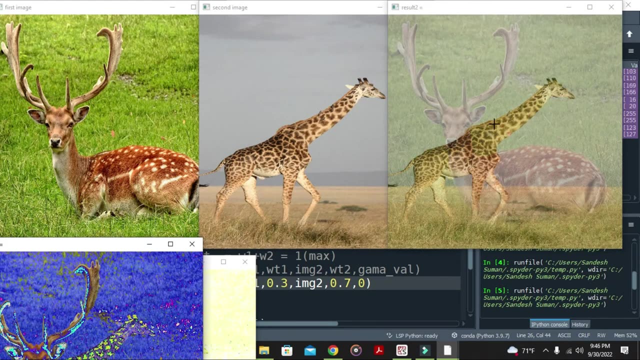 just assign 0.3 here and 0.7 here, then you might notice that your 0 is dominant in the picture. so yeah, you can see that in the result 2, the 0 is more dominant than that of your deer right? so this is what add weight function will. 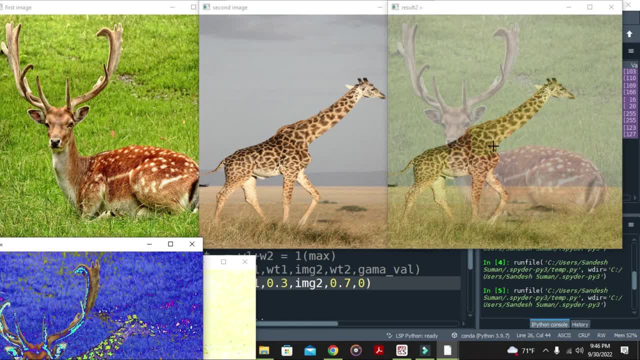 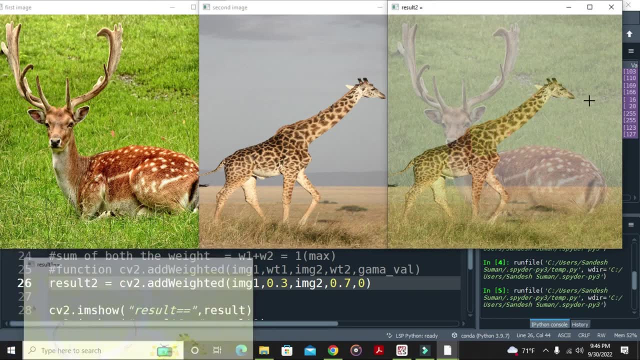 do? it simply adds and adds the weight. right, it simply assigns the weight to your image and that is how you get the blended output and that is how it adds the image. so that was all about image planning. i hope you have understood this. thank you for watching.